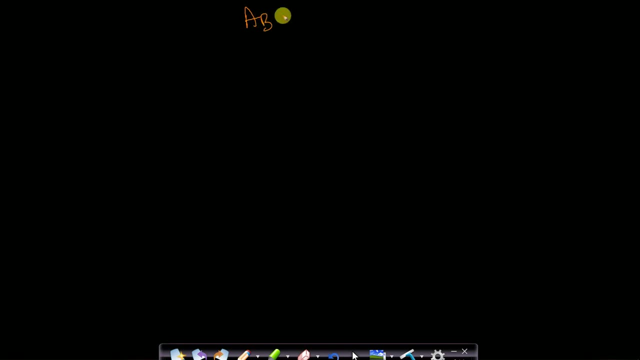 for us to code. Let us take the same example, abc, and try to print all the permutations of this given string. What we can do is we can take this character, a, and we can print just swap it with a. Okay, that means we can replace a with a. Then what will be our string? 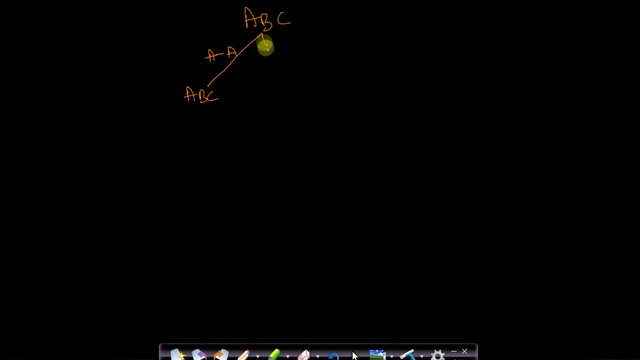 Our string will be unaffected. It will be abc. If we take character a and swap it with b, then our string will become bac, And if I take character a and swap it with c, then our string will become cb and a. Okay, so this will be our string Here. you will now find: 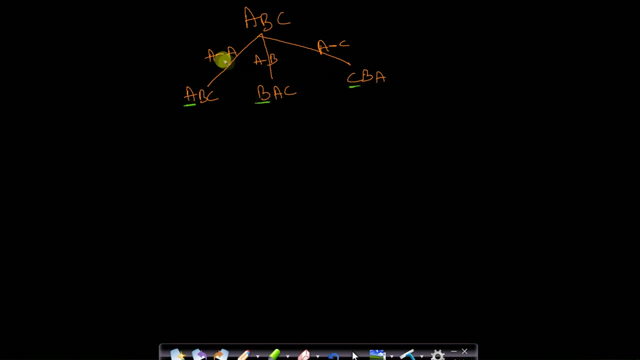 the first character, Since you have always swapped with the first character, so now you will be fixing the first character. Okay, So let us take this abc. In this abc, you have already fixed a, So you can only perform the swap operations between these unfixed characters. 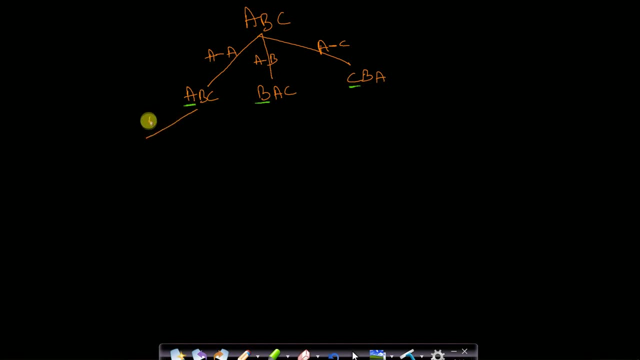 which is b and c. So you have two options left. You can either swap b with b. If you swap b with b, then your string will still be unaffected- abc. If you swap b with c, then your string will become acb. Now coming to bac, you cannot do. 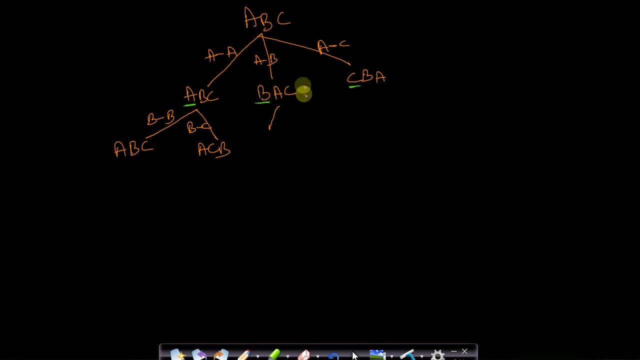 anything with b. since it is fixed Now, you can perform all your operations in a and c. If you swap a with a, then your string will be bac, And if you swap a with c, then your string will become bca. Similarly for cba, you cannot do anything with c If you swap. 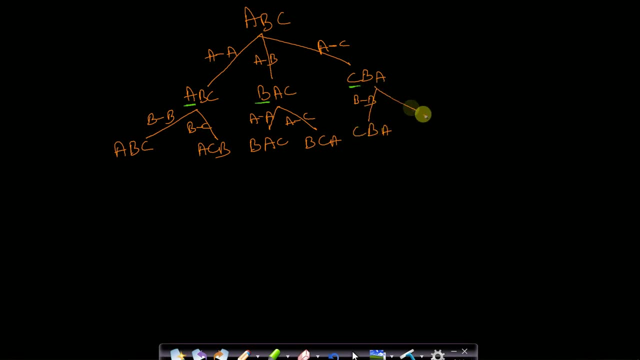 b with b, then your string will be cba and if you swap b with a then your string will be cab. now you can see that your ab, ac, the first two characters will all be fixed, since in this second level, this is, let us say, this is level one, this is level two and this is level three. okay, so in 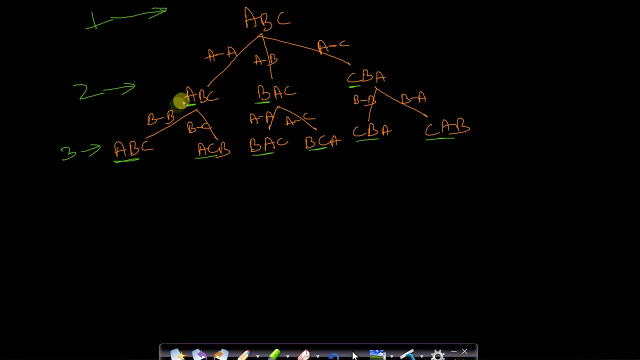 your first level you were just fixing the first character and therefore in the second level your first character is always fixed. in the second level you are always swapping with your second character and therefore in the third level your second character is also fixed. so first two characters are fixed. now, when you have only one character left, then you cannot swap it with any. 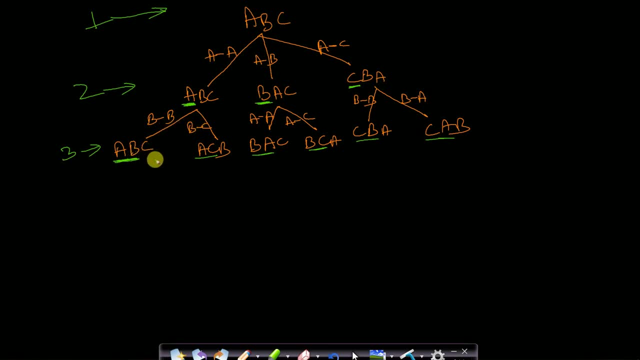 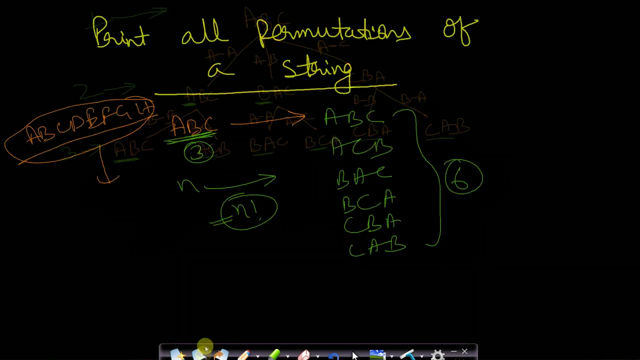 other character and therefore here you will stop now. after stopping, if you can see, you have all the six possible permutations of this ABC. so this is ABC a, c, b, b, a, c b, c, a c b a and c a b, and these are all correct. you can match it with all these six. 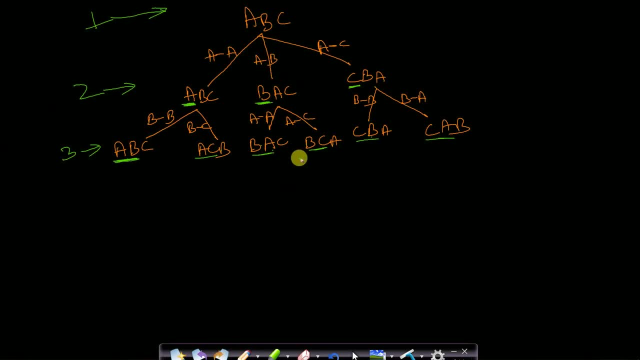 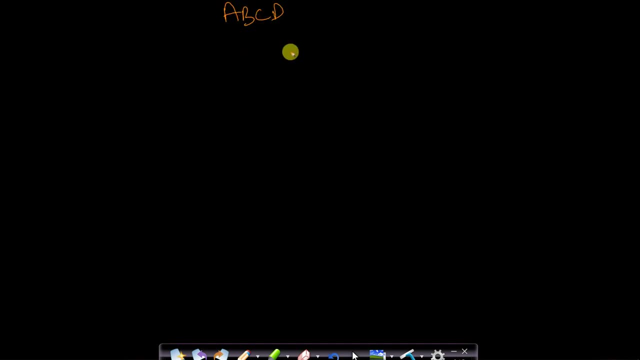 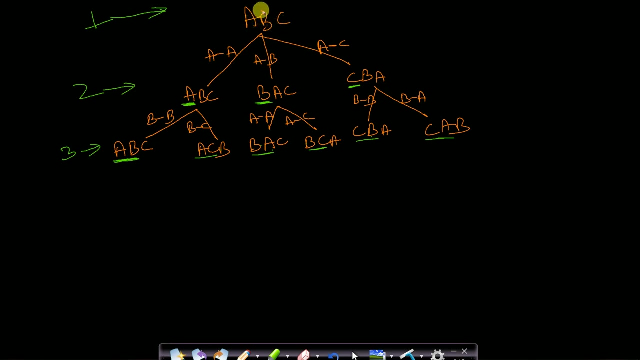 permutations which we have already found. okay, so this is the process. let us take a bigger string and repeat the process. let us take a, b, c, d so that you can better understand it. and, by the way, in this, in this entire figure, if you can notice, the number of characters is always equal to the depth. 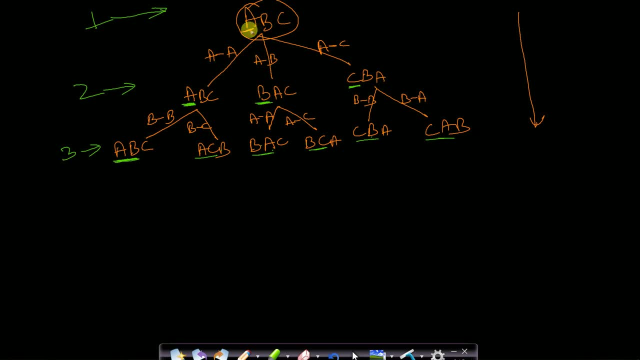 because at each level we are actually fixing a single character. okay, so in the first level we were fixing just one character, so in the second level you can see that a is already fixed, and in the second level we were fixing the first two characters. therefore, in the third level, first two. 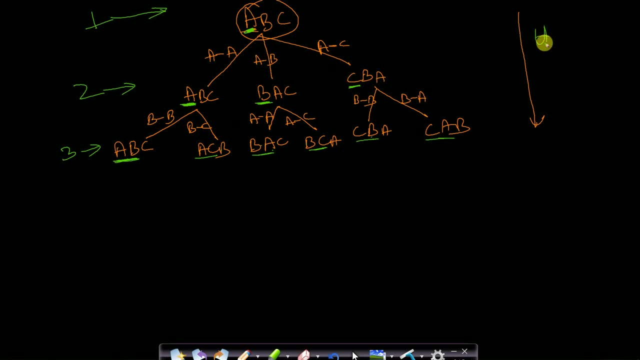 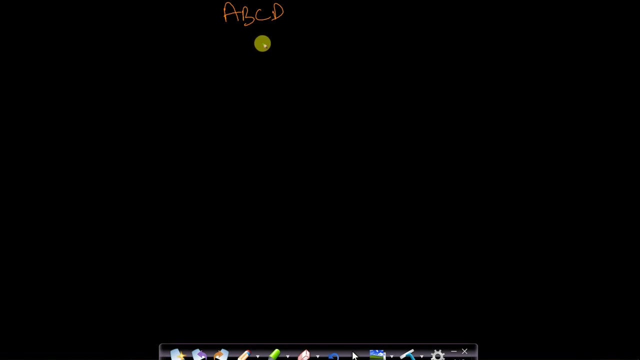 are fixed. okay, so the height of this tree, height, or depth, will always be equal to the length of your length of your string. okay, so this is the very important part of the tree. okay, so now let us go to the next level important point and let us now see the bigger example. let us say: we take a, b, c, d, now what all? 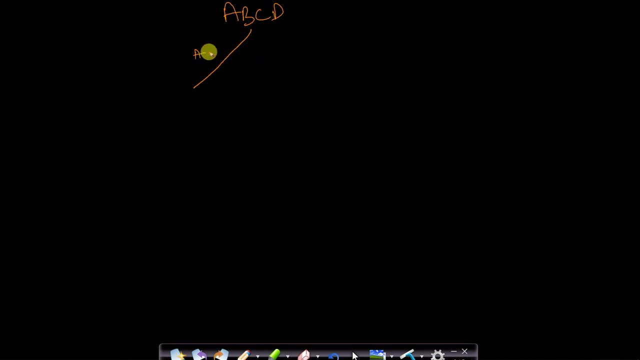 operations can we make? we can either replace a with a, we can do a with b swapping or a with c swapping or a with d swapping. okay, let us say we took a with a swapping, then the string will be unchanged. if we did a with b swapping, then the string will be unchanged if we did a with b swapping. 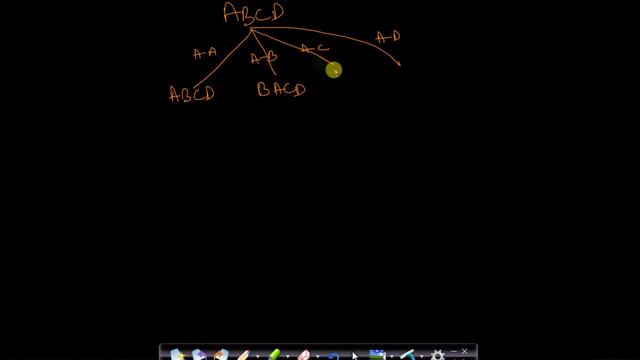 then the string will be b, a, c, d. if we did for a c, then it will be c, b, a, d, and for a d it will be d, b, c, a. okay, now, after performing all these swap operations, the first character of all these strings will be: 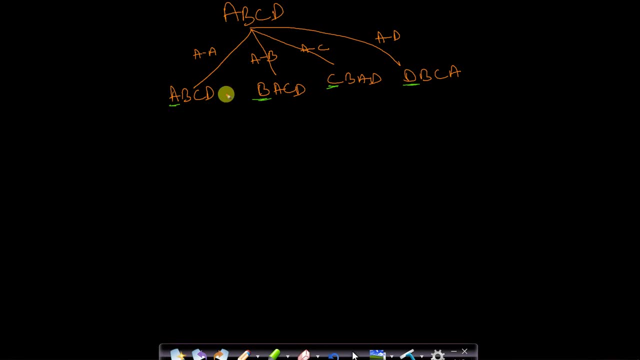 fixed. okay, now, after fixing it, let us see: for a, b, c, d, for a, b, c, d. a is already fixed, so we will do for this: b, b will be swapped with b, or b will be swapped with c, or b will be swapped with d. if b is swapped with b, then the string will 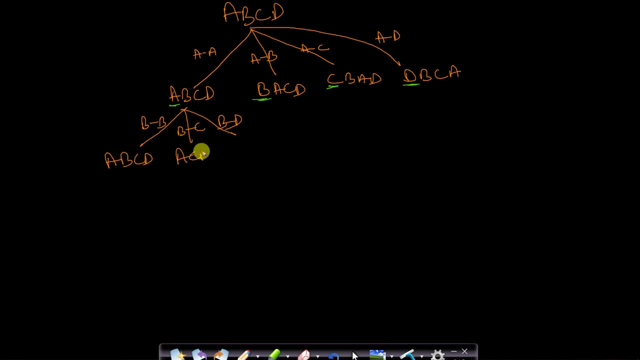 still be same. if b is swapped with c, then it will be a, c, b, d, and if b is swapped with d, then it will be a, d, c, b. okay, so here the first two characters are fixed, because in the first level we were just swapping with the first character. therefore, first is fixed in the first level. this is level one. 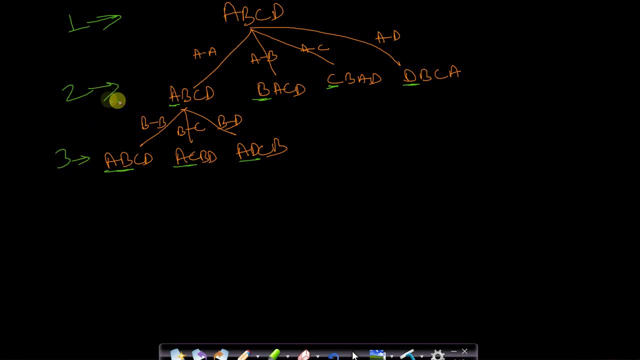 this is level one. this is level two. this is level three. in the second level, we were swapping only with the second character. therefore, two characters were fixed in the third level. okay, and now in the third level. let us take for this a, b, c, d. since a, b is fixed, we will do for c. c can be swapped with. 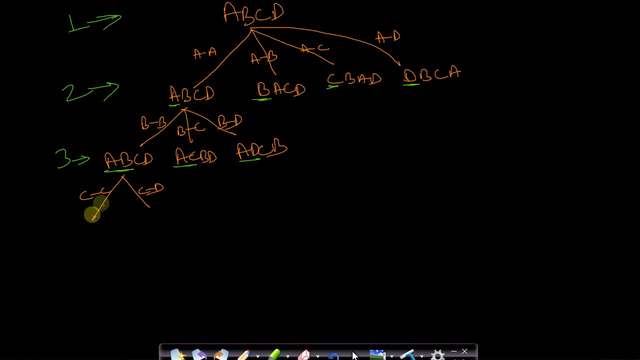 c or c can be swapped with d. okay, so if c is swapped with c, then it will be a b, c, d, string b d, c. okay, and now the fixed characters will be a b, c and a b d. these three will be fixed because in the third level we were doing operation using the third character. we were fixing the third. 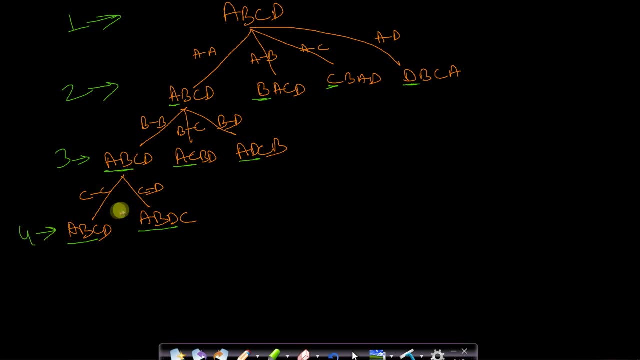 character. so this is level four and, by the way, we can follow this for all these branches. okay, so these will be branched and there will be many such branches, so we can complete this entire tree. and you can see that the height of this tree is equals to the length of this string, which is: 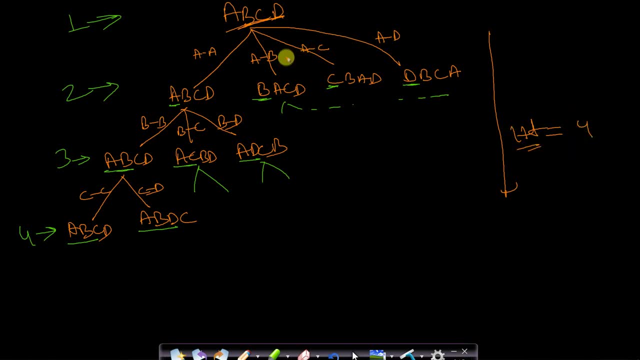 equals to four. okay, and if you can notice, the branching is always decreasing. you can see that at level one we had four branches. why? because the number of positions to which a could have been swapped with were four. and as we are going on fixing the characters in the second level, you 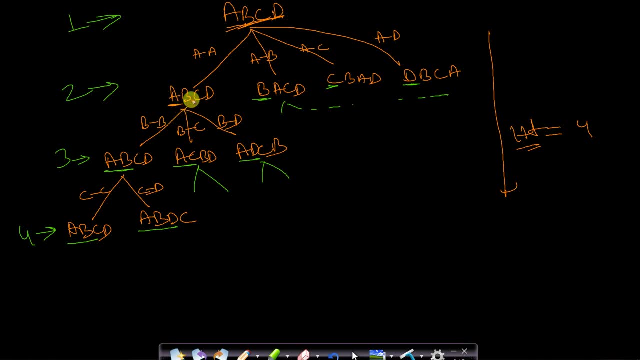 can see that one character position is fixed and therefore the branches will decrease by one. and in the third level, two characters were fixed and therefore the number of branches will decrease by two. so as the depth of this tree increases, the number of branches will also keep on decreasing because we are fixing the characters. 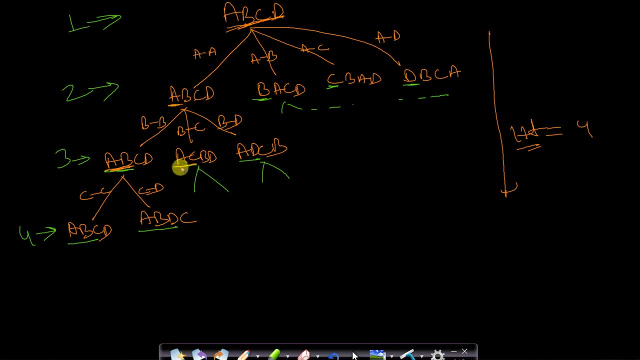 okay, by fixing the characters, we are making sure that we are not allowing swap operations in those characters which are fixed. therefore, the number of possible branches, the possible permutations to be printed will also decrease when we fix the characters. so this is the reason. so we have noticed. 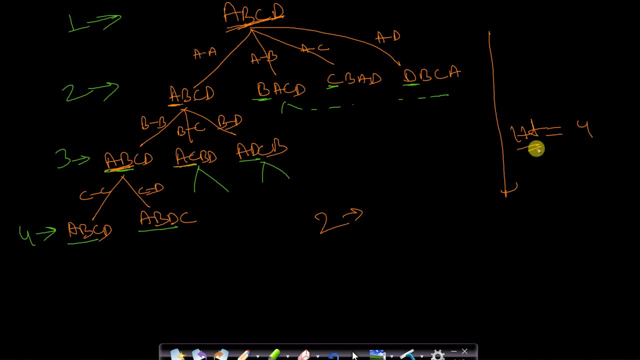 two points: the height of the tree is always equals to the length of the string, and second point is that we have decreasing number of branches as we move down the tree, as we move towards the leaf, and at each level, the number of branches decrease by one. okay, so these are the two takeaways. let us now 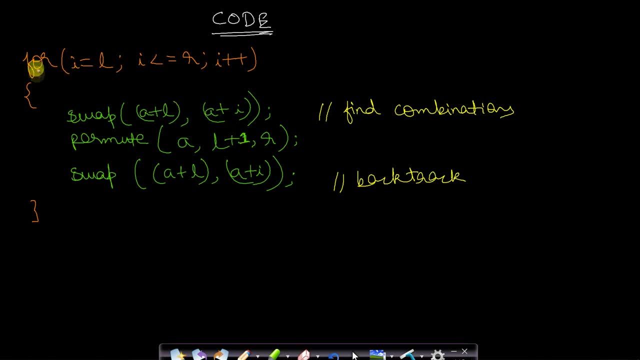 see the code: how to code this. you can see that this is a very simple code and the entire code will be present in the description section below, so please do check it out. the first condition is that if your string is having just a single character- let us say it's a- then it will have only one combination and and therefore, if 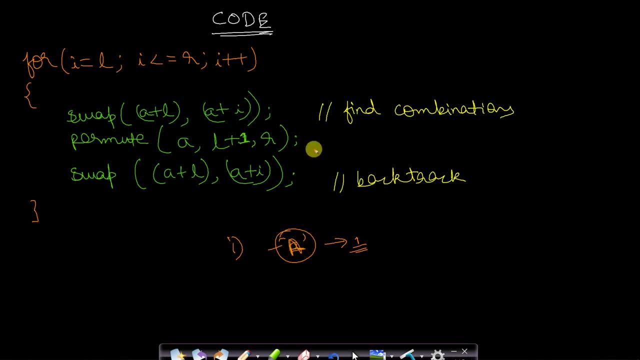 your string only has a single character, then we will just return without performing any operation, okay. but if your string has more than one character- in our case it was say a, b, c- then we will not just return it, we will have to perform all the operations, these three. 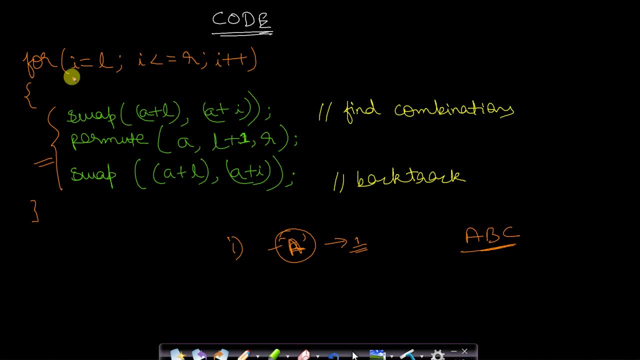 are our operations. okay, what we are doing is we are taking a loop which is equals to low and high. here I have taken left and right. okay, so let us assume that these are our indices and initially the left value is zero and the right value is two. now what we will do is we will run our 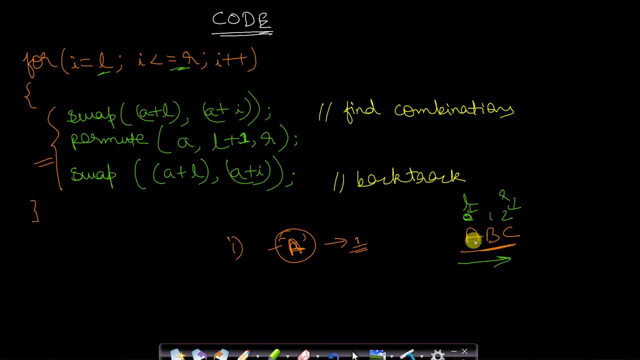 loop from low to high, that means from left to right, from zero to two. taking this zero, what we will do is we will just swap this a plus l with a plus i. okay, so l value is zero and i value. since we are starting it from l, it will initially be zero. therefore, what we are doing is in the first 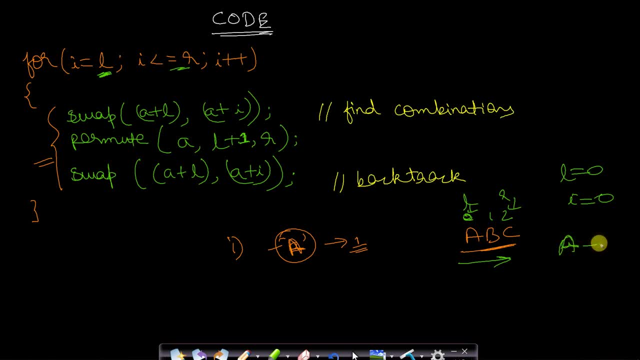 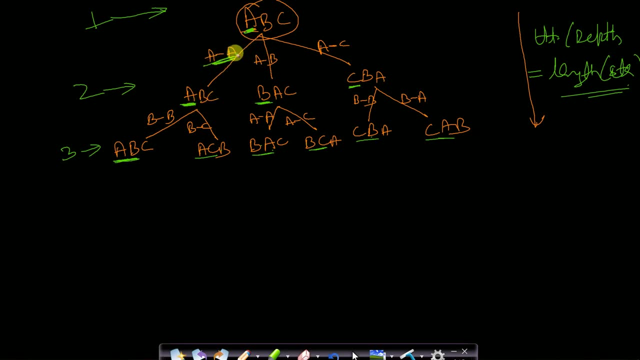 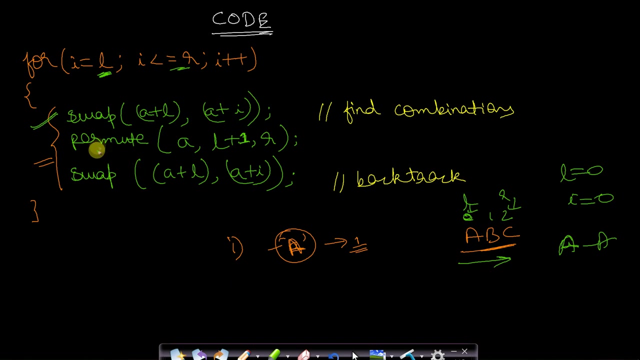 loop, we are swapping this a with itself, and this is what we were doing in the first loop, in our first branching. you can see that we were swapping a with a and therefore the string came out to be same. this is what we are doing in the first iteration. okay, after doing this, we are 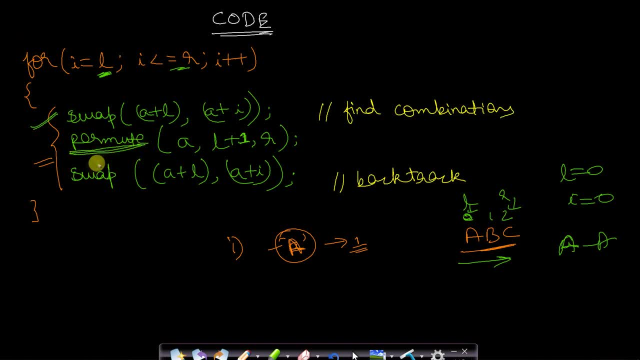 calling this recursive function. this for loop is inside the function permute. we are calling a recursive function and we are trying to calculate all the possible permutations by fixing the first character. we are passing this low value as l plus one. why? why are we doing this? because we want all the possible permutations to be found by using all 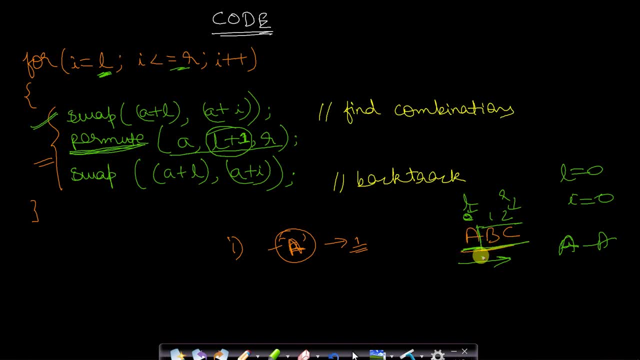 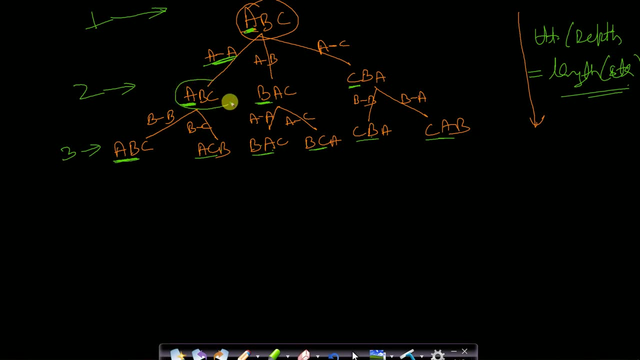 the characters. after fixing this first character, we are actually fixing it. so in the diagram you can see that we were fixing this first character and after fixing the first character, all the possible combinations will be here, only two. it will be a, b, c and a- c- b after fixing a. okay, so 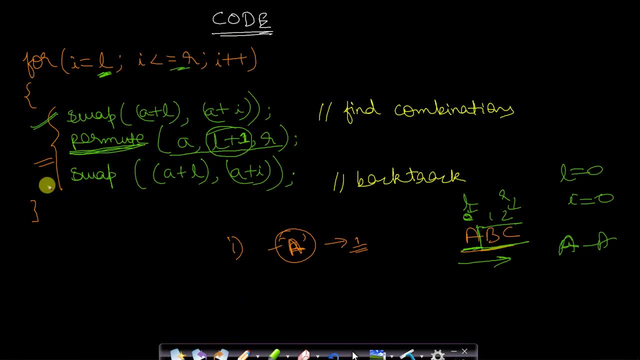 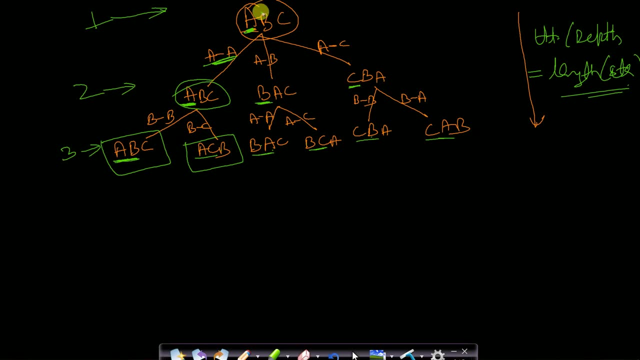 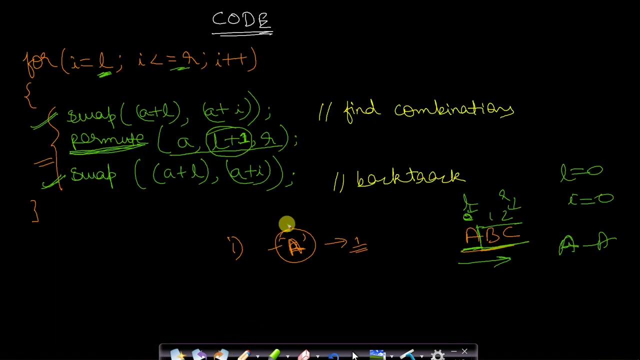 this loop is trying to find all those combinations. this third line is actually used for backtracking. why? let us see the example. we were just printing all the combinations using a single string. so what we are doing here is in our code. we are actually modifying the same string. okay, so when we come back, let us say we are following. 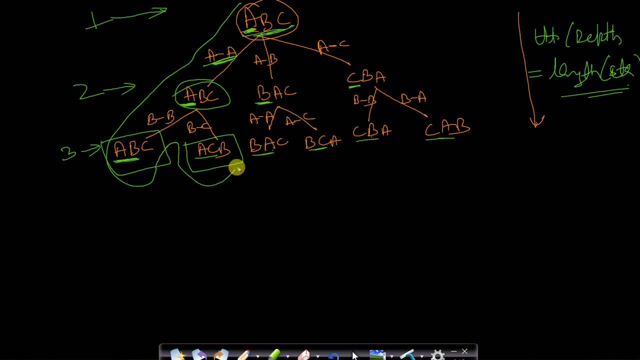 this path and we printed a b, c and then is a c, b, okay, and we came back to a b, c. now, when we come back, when we printed a b, c and then printed a c, b, and when we go back after printing this a c, b- 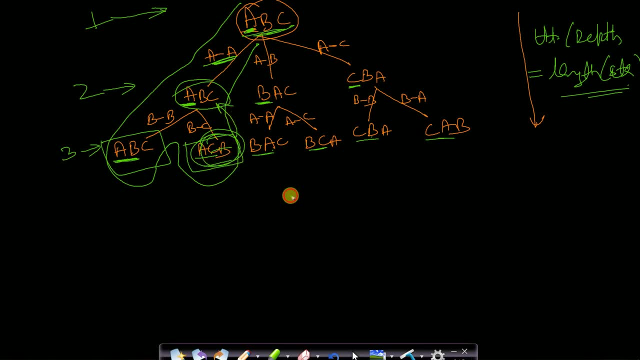 we go back to, let us say, a b c, then we want to rearrange this acb to a b c. okay, so that the next time we can permute this a b c to b ac. we cannot directly go from acb to bsc. we will have to follow the path from a c- b to a b c and from a b c to again. 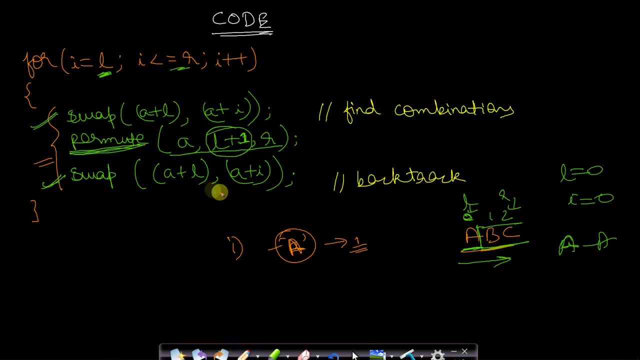 BAC. okay, so that is why, in order to recover our original combination, the original permutation which we had, we will again use the swap operation, which will cancel out our original swap operation. okay, let me give you an example. let us say: if you have ABC- okay, you swapped A with C- then what will? 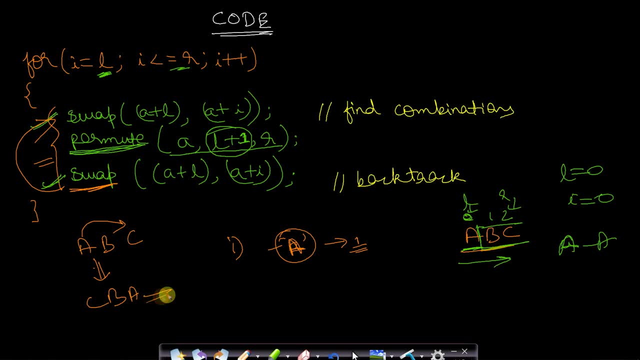 be the result? it will be CBA. and again, if you perform the same swap operation, if you swap this first with the last, then it will be ABC. this is what is happening here. you can see that our original string was ABC and our recovered string is also ABC. here I had performed the swap operation. 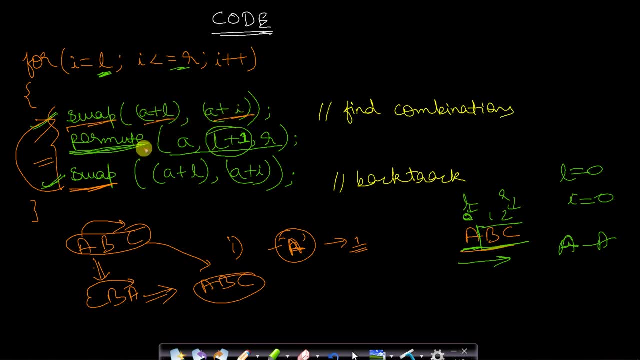 using A plus L and A plus I, and after printing all the permutations using this combination, I am just recovering our original string by performing the same swap operation- A plus L and A plus I, which will recover our original string. if you find any difficulty in the code, then 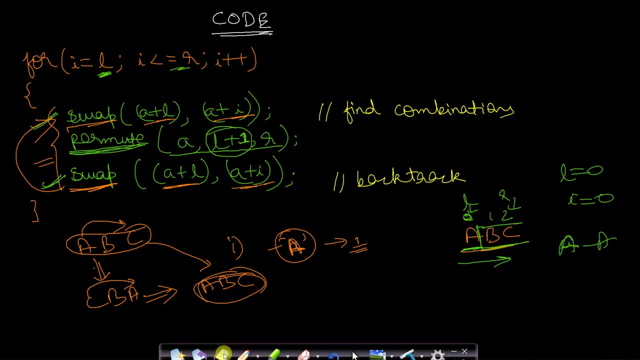 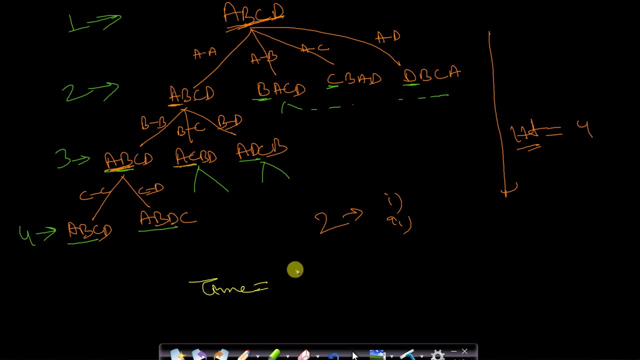 feel free to comment below and I will try to help you as soon as possible. so let us now look at the time complexity. now, what will be the time complexity? the time complexity will be order of time to print. time to print only one permutation, time to print only one permutation, and that will 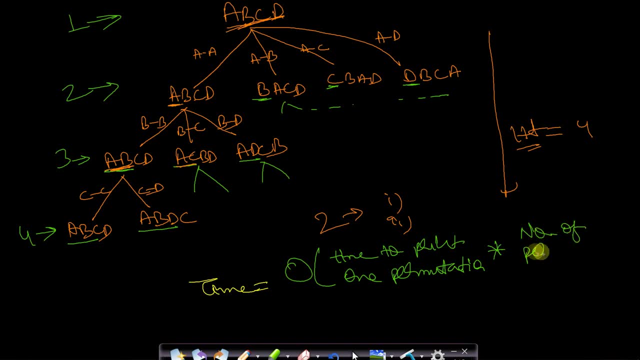 be multiplied with the number of permutations. okay, so this will be the time complexity. so you can see that if you have a string ABCD, then the depth will be order of n. here n is the length of string, and let us say it is four. then, in order to print just a single combination, you can see that. 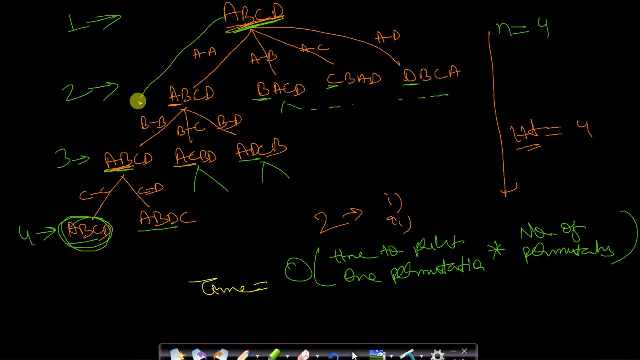 in order to print this ABCD we had to traverse through a depth four. so in order to print only a single permutation, the time will be order of n. okay, that will be equals to the depth of the tree, and then the number of permutations possible with a string of length. n is n factorial, so that will be multiplied with. 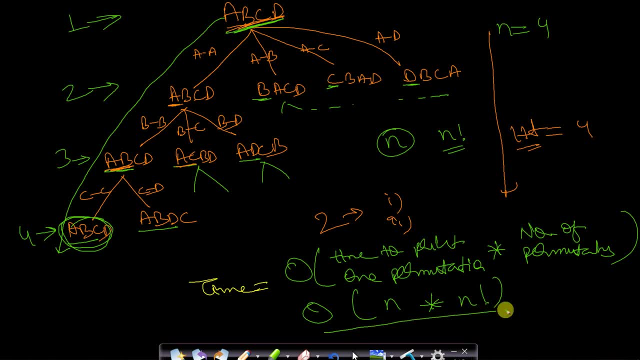 n factorial. so the total time complexity will be time to print one permutation from the given string, which will be order of n multiplied with the number of permutations possible with a string of length n, and the total time complexity will be order of n into n factorial. I hope you were. 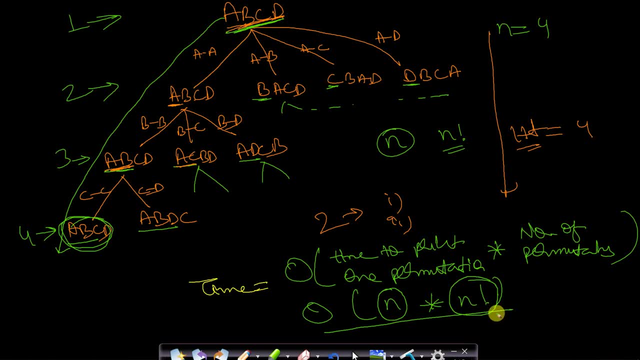 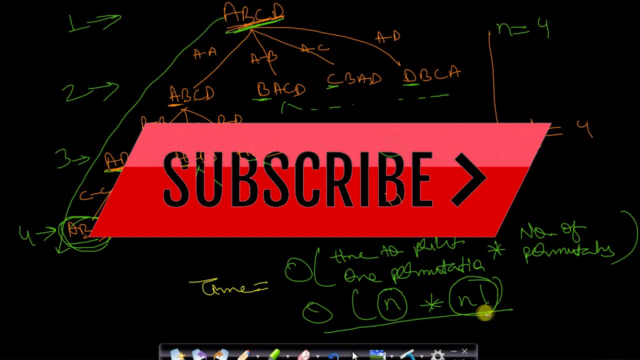 able to understand how to print all the permutations from a given string. if you find any difficulty, then feel free to comment below, like and share our video and subscribe to our channel in order to watch more of these programming videos. see you in our next video, thank you.